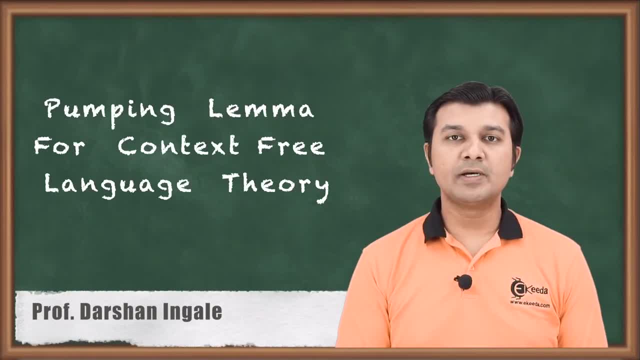 Hello friends, welcome to the next chapter. Over here we are going to study how do we write the pumping lemma for context-free language. First and foremost thing, let us understand why do we require a pumping lemma now? So let's get started in this topic. 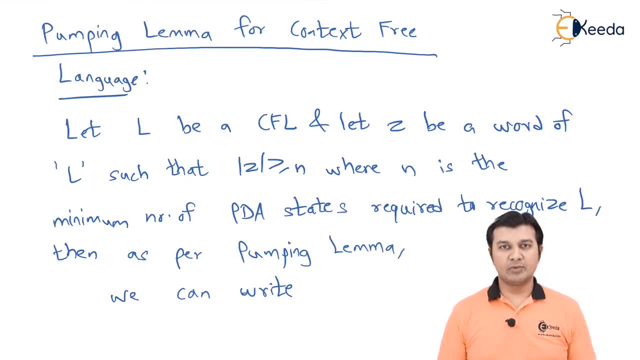 So now, friends, we have already seen what is Turing machine and we know what is the importance of Turing machine. All the problems which cannot be solved using pushdown automata- that is, the language of pushdown automata, which is context-free language- All the problems which are not getting 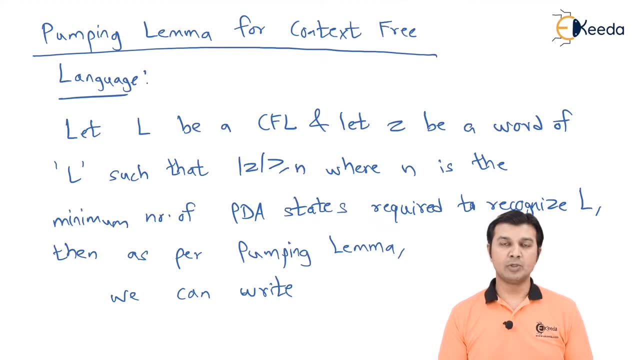 solved by PDA are solved using the Turing machine. So, friends, why do we go for Turing machine? Because, with the help of pumping lemma, we are able to prove that some of the problems cannot be solved by PDA. So how are we going to prove that a language is unable? 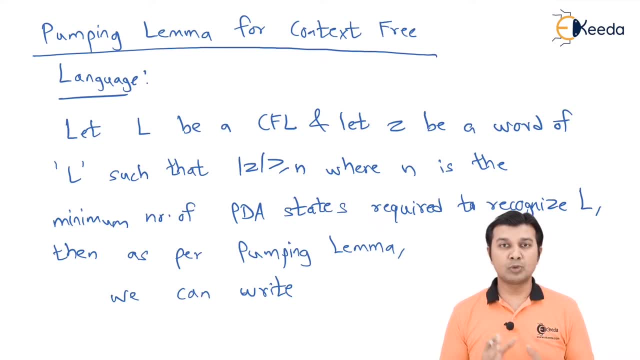 of solving, or how do we prove that a pushdown automata is unable to solve context-free language? that is, with pumping lemma Again over here we are going to use the hypothesis assuming that it will be able to solve, which, at the end, by contradiction, we prove that the language is not context-free. 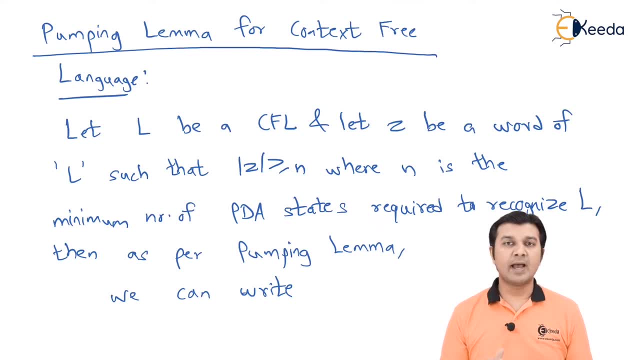 language and therefore pumping lemma, is going to reject that, and hence we go for new type of machine, that is, Turing machine, to solve this problem. So, friends, let's understand the pumping lemma. now The pumping lemma over here is again tricky. So, as I advised you previously, pumping lemma for regular language, wherein you have to remember a certain 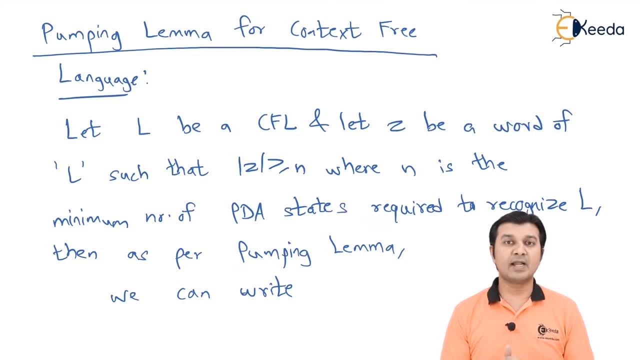 set of steps and only do the mathematical steps that are going to change. in every problem. The same thing is going to be true over here. So initially you might find the definition a bit weird, but trust me, it is the way you have to write and only some of the calculations are going to. 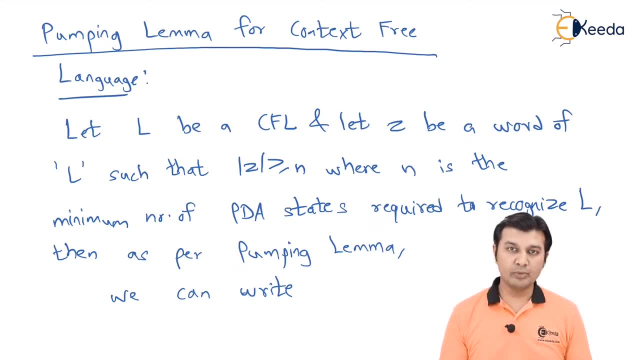 change in all of the problems. So let's understand the pumping lemma now. The pumping lemma over here is going to help us solve these problems. So therefore, how do we define it? The pumping lemma for context-free language: Let L be the context-free language and let Z be the word of L. that is any string of that. 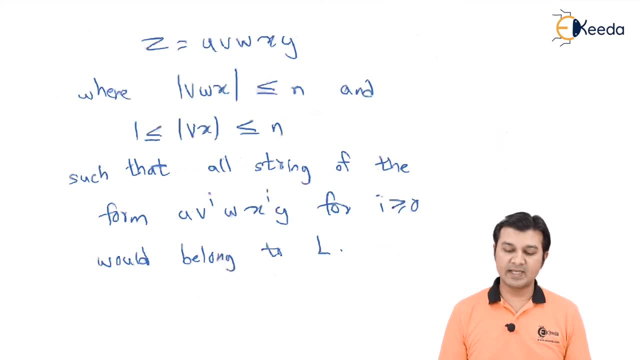 particular language such that mod of Z is greater than equal to N, where N is the minimum number of PDA states required to recognize the language. Then, as per pumping lemma, we can divide this string into five different parts. Therefore we write: Z is equal to UVWXY, where mod of VWX less than equal to N and 1 less than equal to mod VX less. 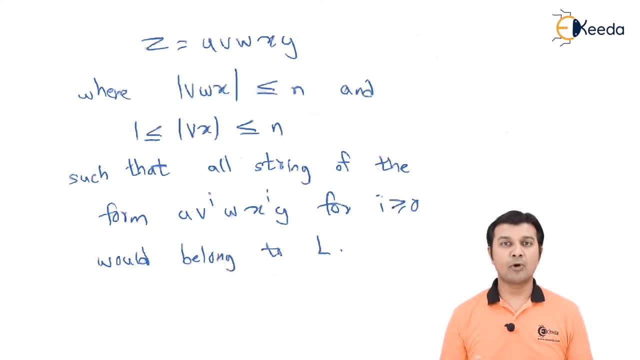 than N. From how did it came? It came from a theorem which we are not discussing because what comes in the exam is the problem. So we have to assimilate the theorem as it is, assuming the things are right, Such that all the strings of the form U, V raised to Y. 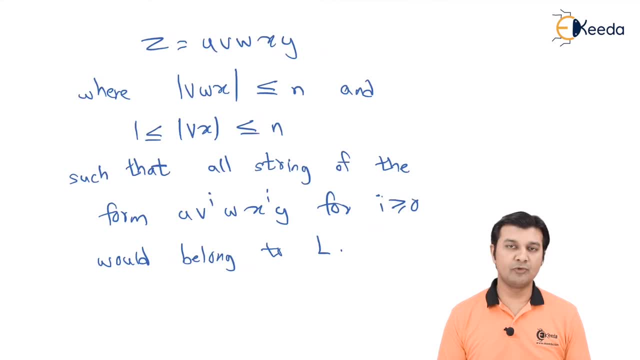 W, X raised to Y, Y for I greater than equal to 0 would belong to the language Friends. previously it was X, Y raised to Y, Z for pumping lemma for regular language. Now, over here, the entire string is divided into five different parts. So, friends, using this particular theorem, we are going to 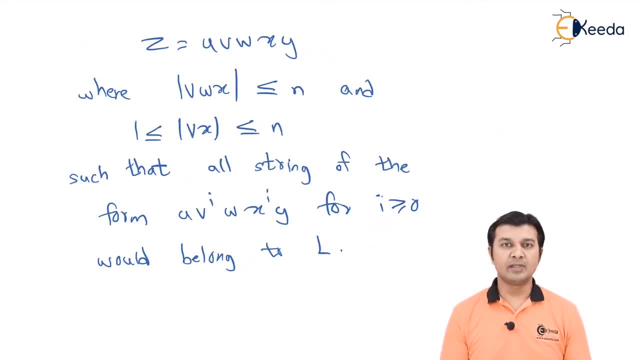 solve two problems on the same and prove that pumping lemma for context-free language is able to prove by contradiction that the language is a context-free language. So we are going to solve two problems. which is not CFL and therefore PDA cannot be used for recognizing it. So with this, 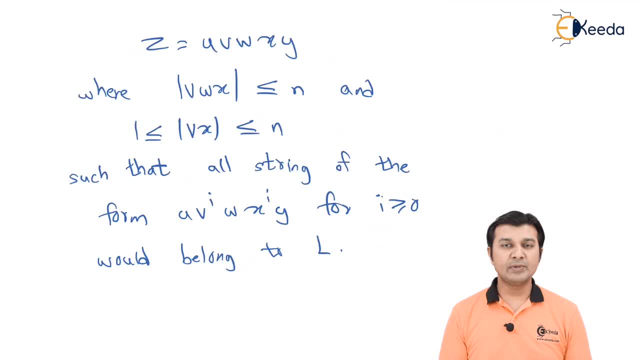 we stop with the definition of pumping lemma and see you in the next session, where we will be solving the problem on the same and throwing some more limelight on the definition. Thank you, friends. 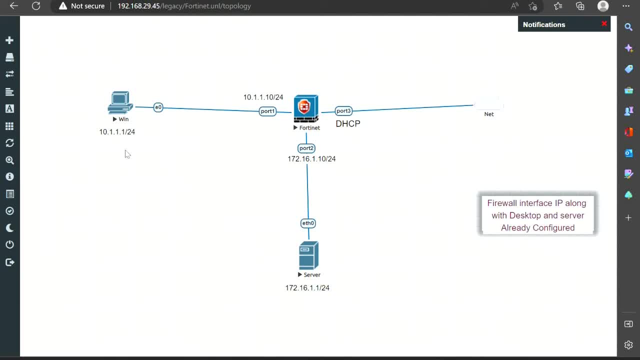 hello guys, welcome back once again. today we are going to learn that how to configure firewall policy on the 48 firewall. all right, so for this lab demonstration, i have one 48 firewall here. this is our dmg server and this is will be, we can say, our machine. and but for the real life, 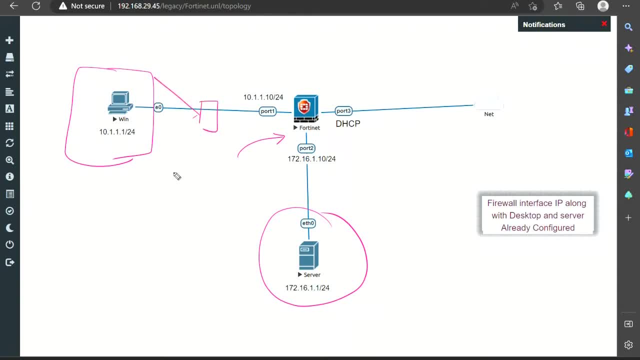 example, you can take it as like a switch here and multiple machines connected here. but i have not taken switch, just for the simplicity, just one computer connected, but the environment can be like that, one for the complex scenarios, right. so, and this part is our internet, so this interface.